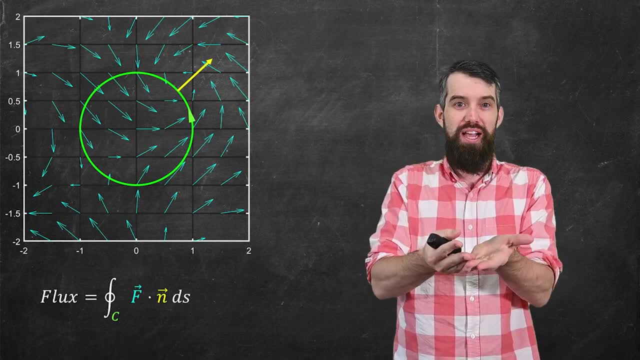 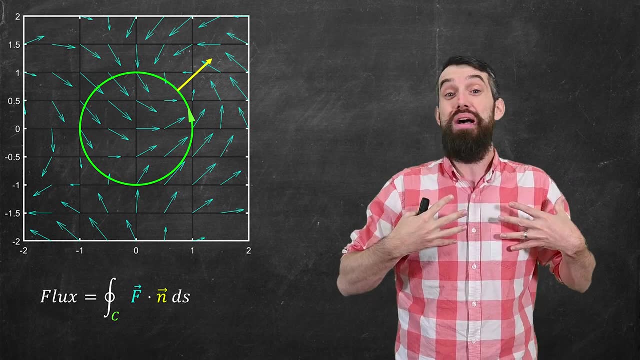 field f at a particular point that was pointing normal. If the field was just tangential along the curve, then there would be no crossing of that boundary. But if we want to know well how much is stuff crossing the boundary, then f dot n gives us a. 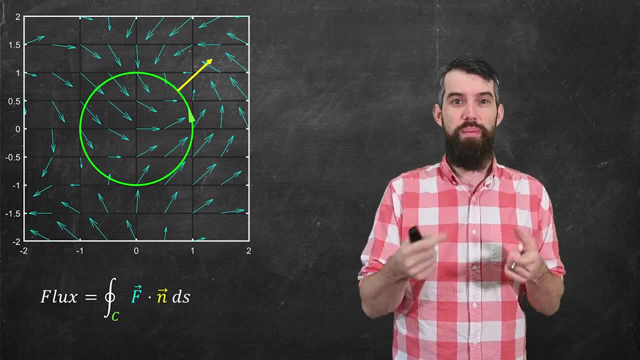 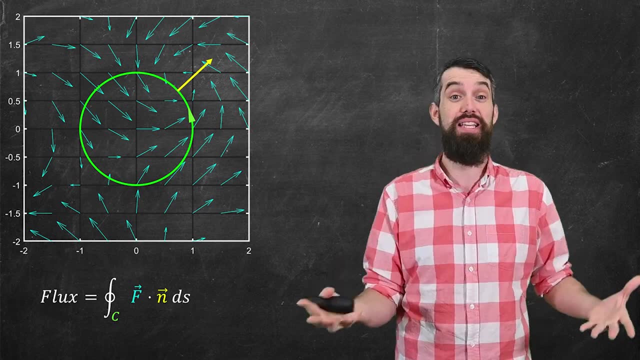 measure of that. And it's important to note here that I'm talking about the outward flux going out of this particular closed loop that I have, in contrast to what could have been defined as the inward flux, which is the portion coming inward. So our n is defined to be an outward normal, That's. 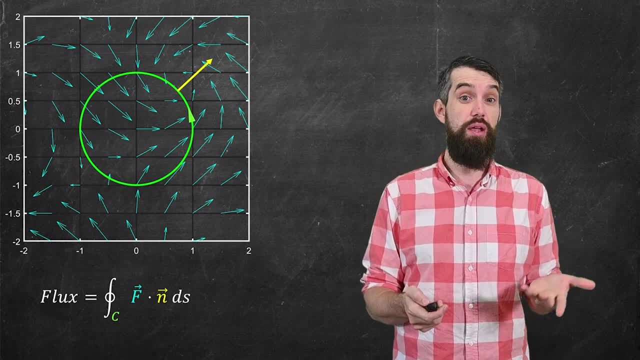 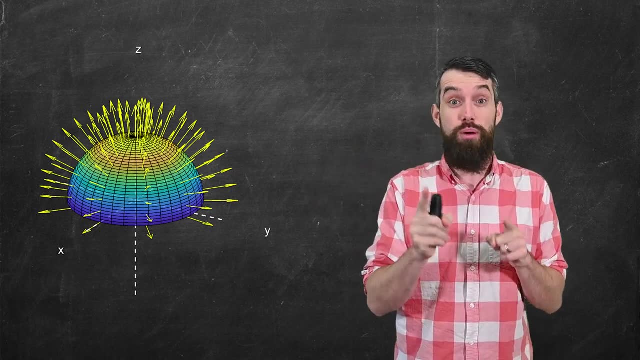 going to be important in a moment. So that's the story with the curve, but it's actually the same thing when we return back to the story with surfaces. What I've done here is not put the vector field up yet. That was going to be drawn in blue. The arrows that you see here refer to the 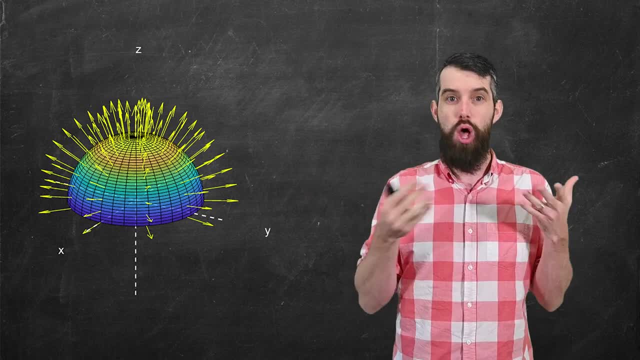 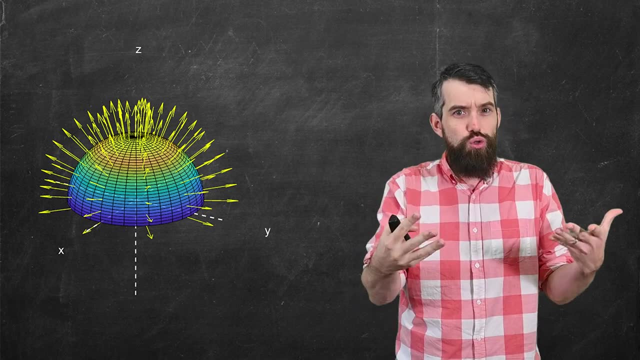 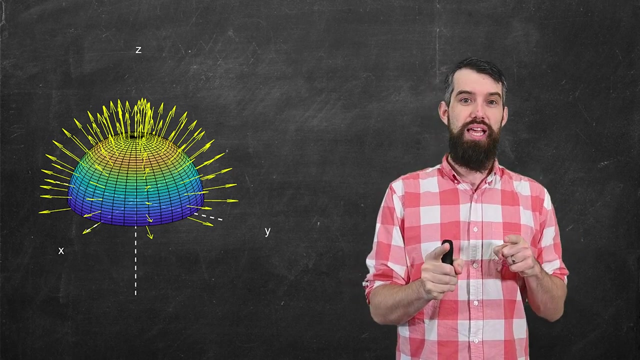 normal vectors to my surface, the top half of a sphere, That is. at any point along the surface there is some normal vector which is pointing outwards from the perspective of the origin, and I've just gone and plotted a whole bunch of those arrows. Now what's key here is that this surface 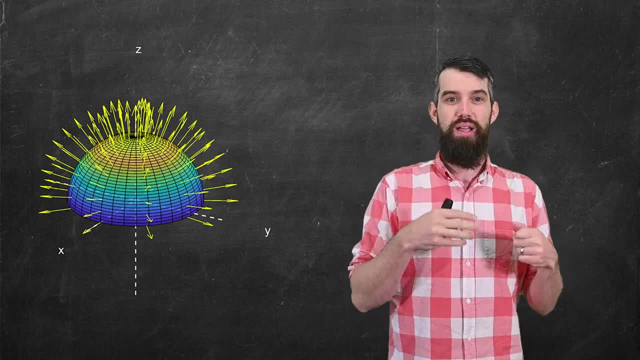 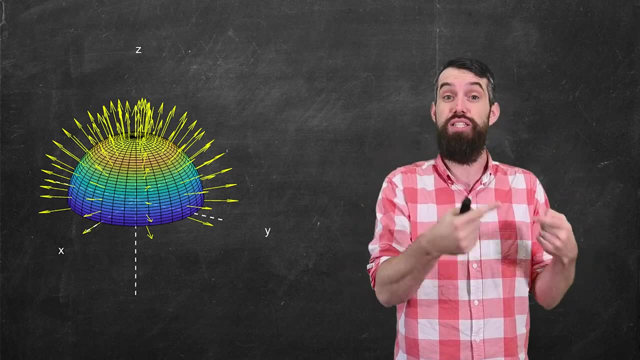 is what we've called orientable in our previous video, And because it's an orientable surface, which means there's two different sides that I can continuously assign these normal vectors to, I have to make a choice, And so I've made this choice where the vectors are all going out from. 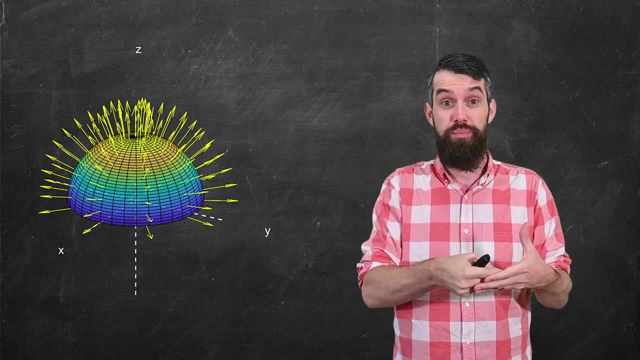 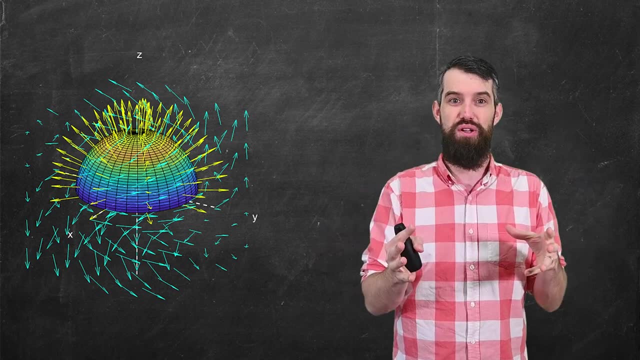 the origin, as opposed to all going inwards towards the origin. And then if I put the vector field back on where I've got now blue arrows, that's the underlying vector field. For example, it might be representing movement of I don't know, say, a compressible gas that's swirling around The. 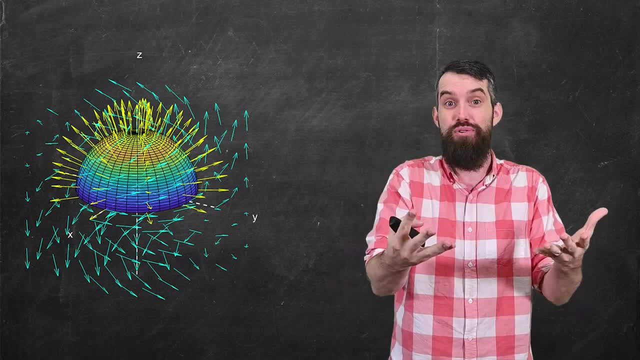 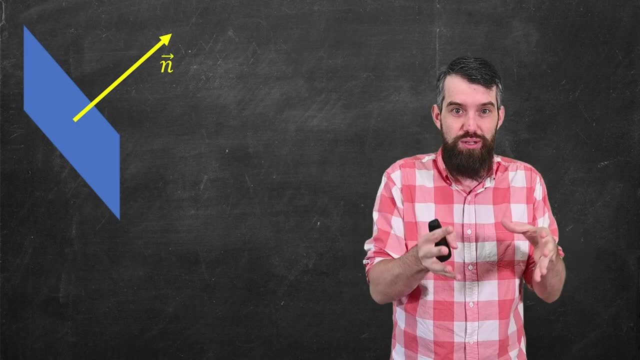 question is: well, how much is that gas crossing the boundary in this outward direction? So if I zoom in really closely on a small portion of that surface- so I've got the small surface and I've got the normal that I put here- then my 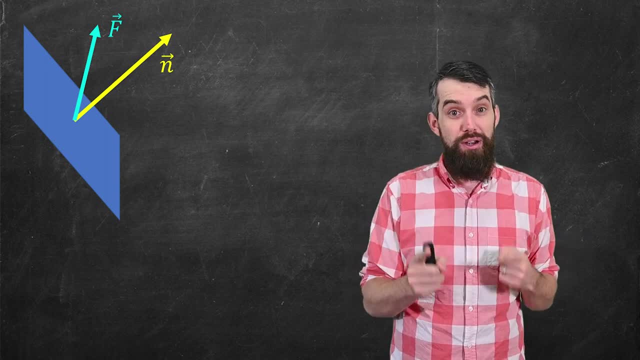 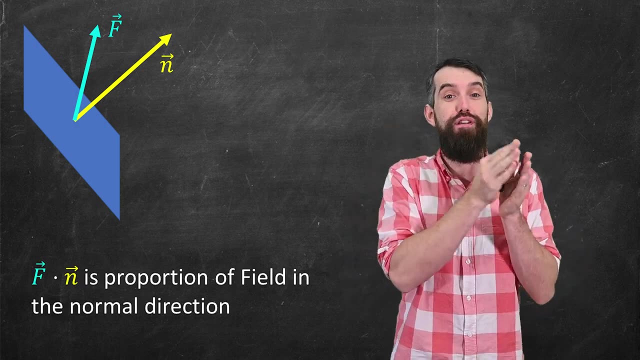 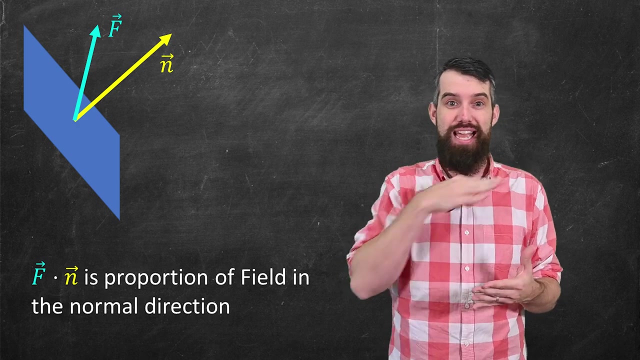 vector field is just going to be well, some vector. So what I'm interested in is measuring f dot n, because f dot n is going to be the proportion of the field which is in that normal direction. If the f vector lay in the surface, if it was tangential to the surface, 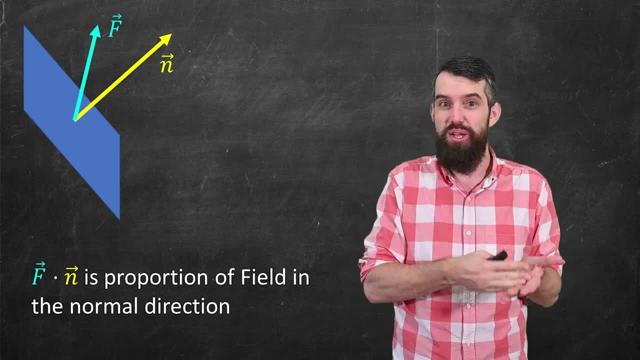 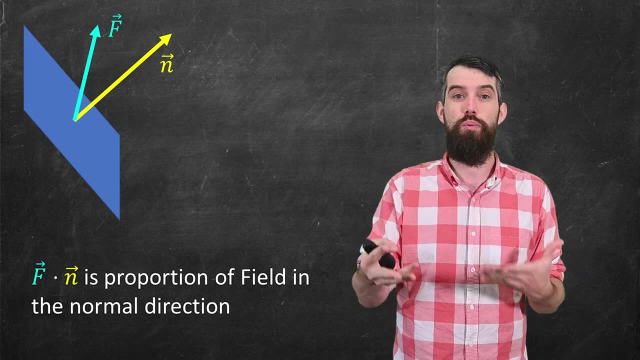 then there would be no crossing of the surface at that particular point And f dot n would be zero in that case. But generally, f dot n tells us the proportion of the field that's in the normal direction And, as a result, if I want to know the total flux over the entire surface, well, let's. 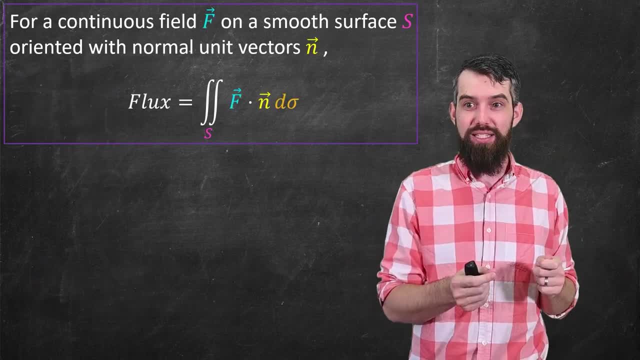 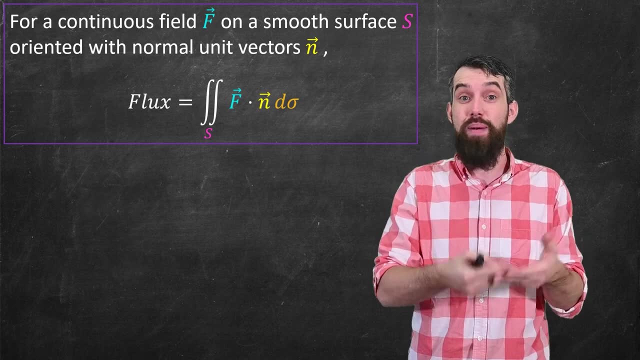 just do a surface interval. I'm going to say that the flux is, I just integrate f dot n over the entire surface. In other words, it's integrated d sigma. d sigma is my little element of surface area. My assumptions are that I haven't thought about that. 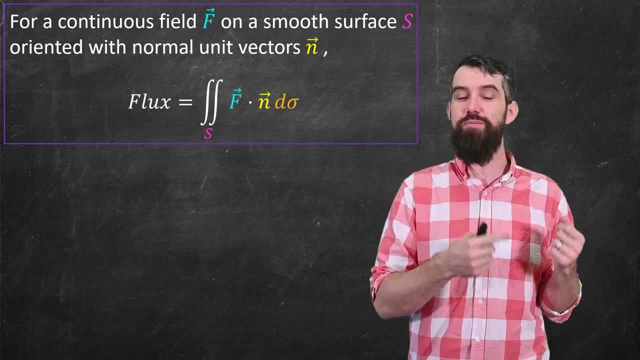 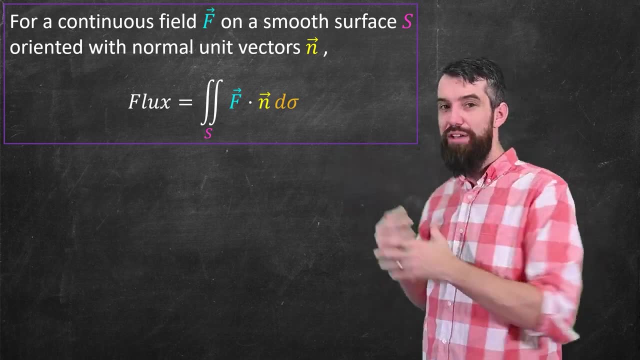 So I'm going to use the surface area as the vector field f, together with a smooth surface s that's being oriented in some way by the normal unit vectors. Now, as we do over and over in vector calculus, we come up with some definition that makes good intuitive sense to us in terms of ds. 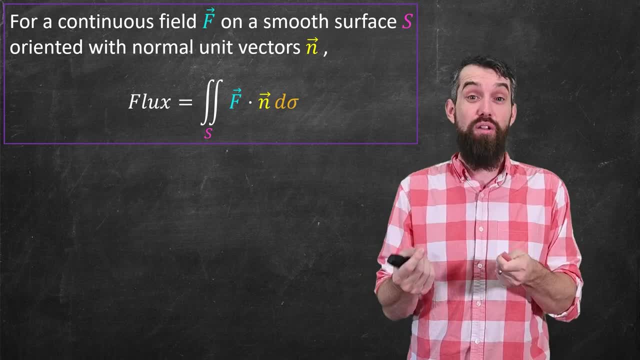 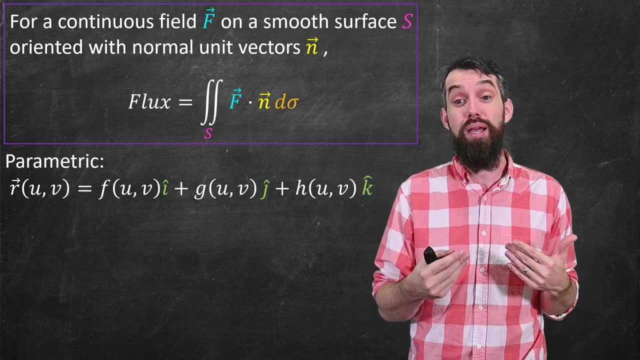 or d sigma, but then we always had to find a way to compute it depending on the way the underlying surface or curves are actually described. So first let's consider what happens if my surface is described parametrically as a position function of u and v in its three different components. 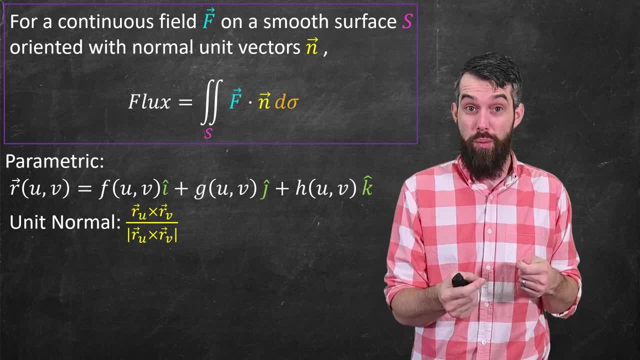 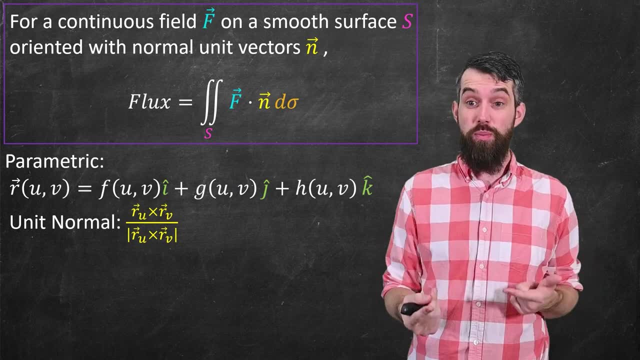 Well, one of the things we've seen before is that a choice for the unit normal is ru cross rv over the length of ru cross rv, And so I'm going to imagine that, if my surface is orientable, that I'm choosing this particular set of unit normal vectors versus the negative, which also could have been possible. 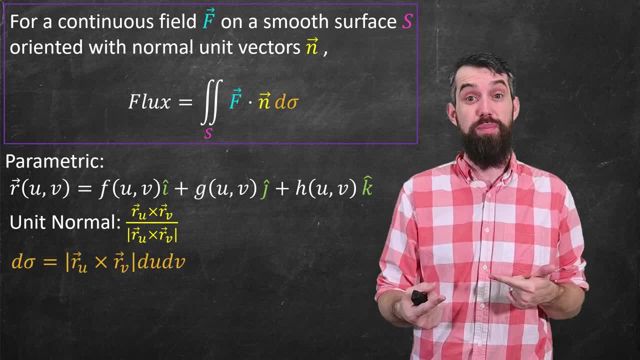 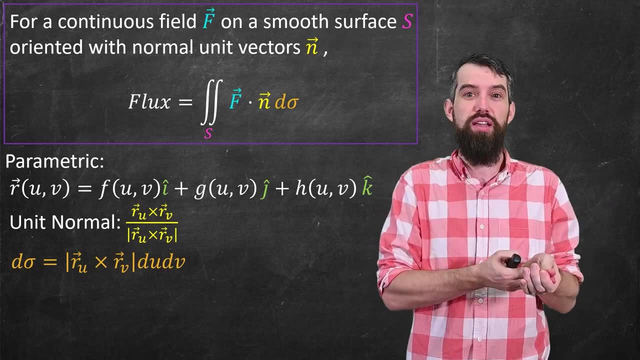 Similarly we've seen before that for a parametric description the little element of surface area can be described d sigma as the length of that crossbar, the length of ru cross rv and then times the length of ru cross rv. So putting this all together, what is the flux? Okay, it's the f dot n. I've substituted. 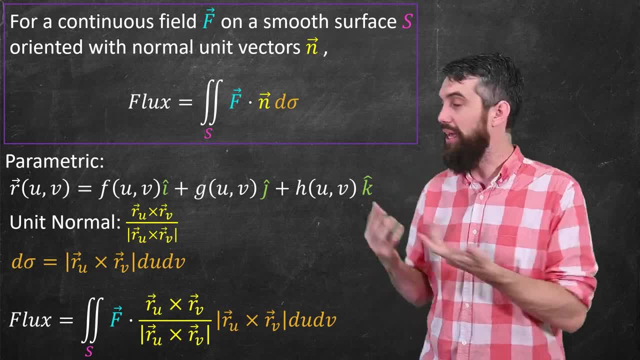 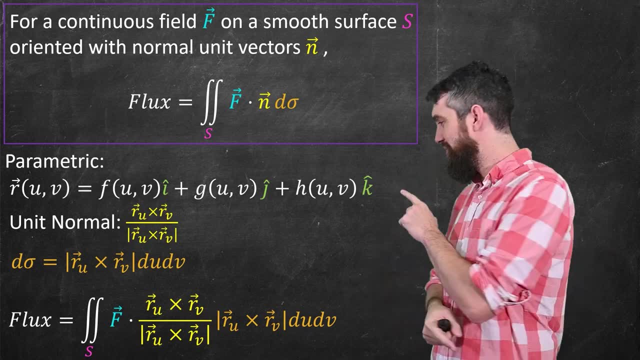 in the unit normal that I just talked about, and then the d sigma is being replaced by the ru cross rv, its length d u d v as well. This looks messy, but at least there's a simplification. I see that there's a length of that ru cross rv in both places, so I can cancel that from the top and the.